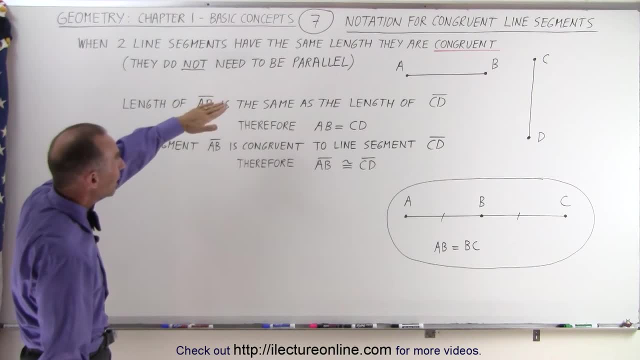 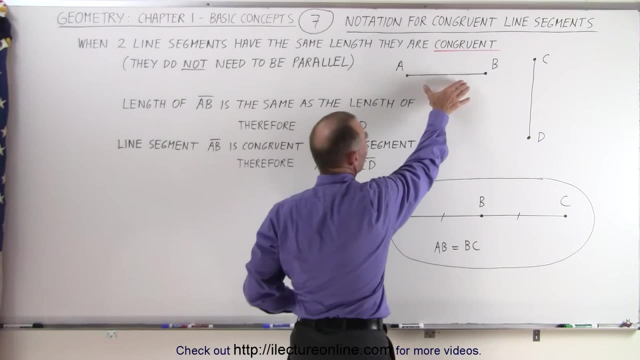 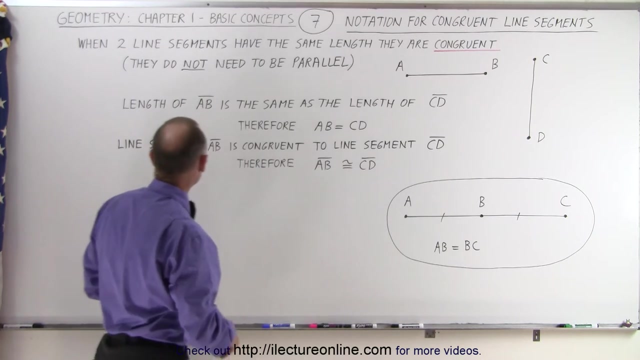 do we use? So when two line segments have the same length, we call them congruent. They don't need to be parallel. So here we have a line segment AB and a line segment CD And by inspection you can see that, yes, they appear to have the same length. So if the length of line segment AB 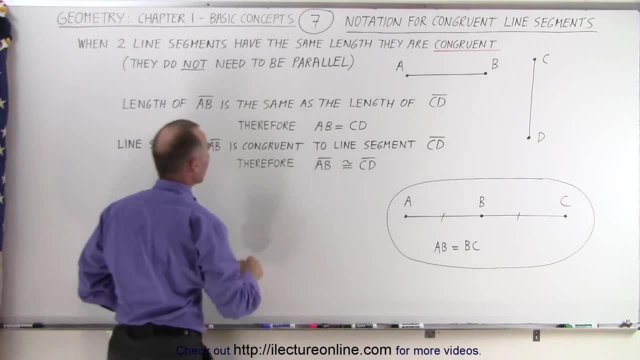 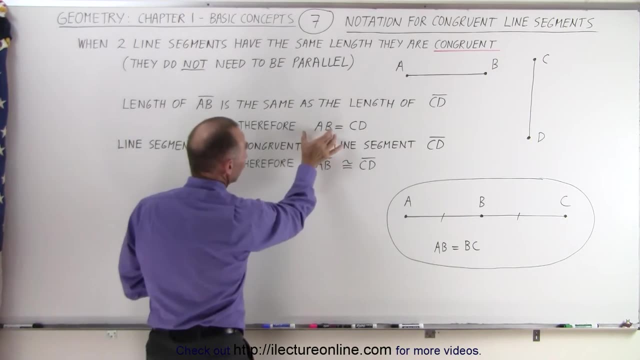 is the same as the length of line segment CD. we can then claim that AB equals CD. So when we write it like that, we mean the length of line segment AB equals the length of line segment CD. AB indeed represents the length of line segment CD. 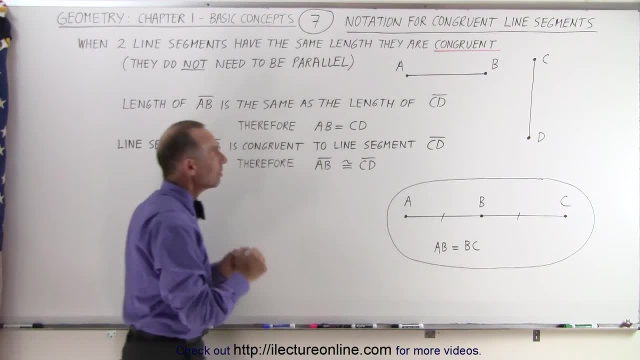 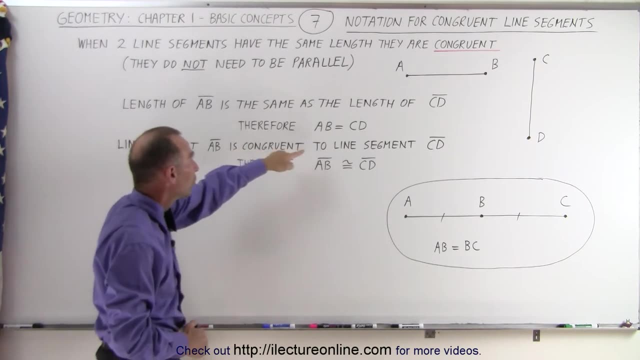 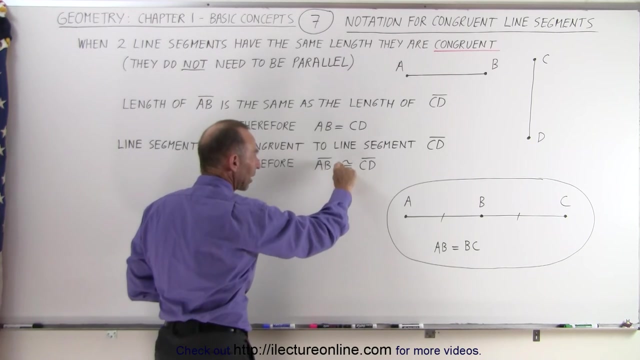 Between A and B, and CD represents the length between C and D. However, if we write it like this, the line segment AB is congruent to line segment CD. then we can say that the line segment AB. we write an equal sign with a little squiggle line on top, the line segment CD. This symbol here. 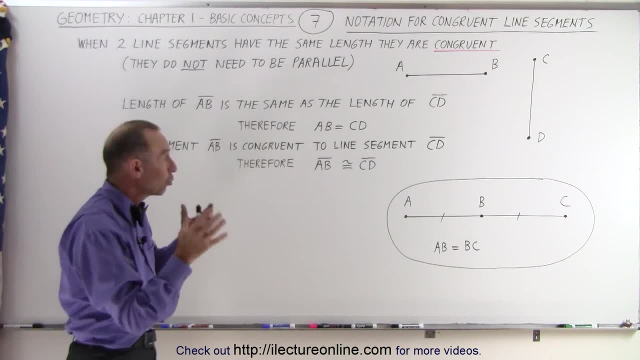 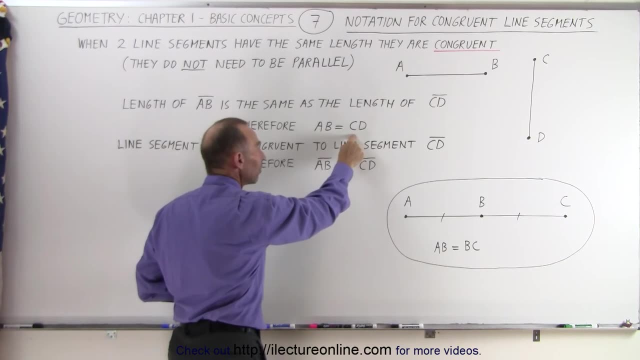 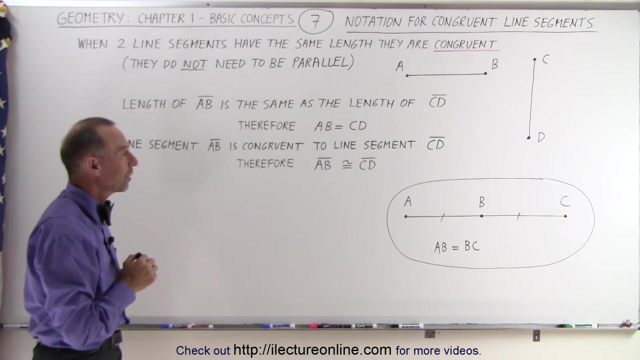 means congruent, and that simply implies that those two line segments have the same length. Here we basically write that the length of AB is equal to the length of CD. The length of line segment AB is equal to the length of line segment CD. Subtle differences: different notation, Another way in: 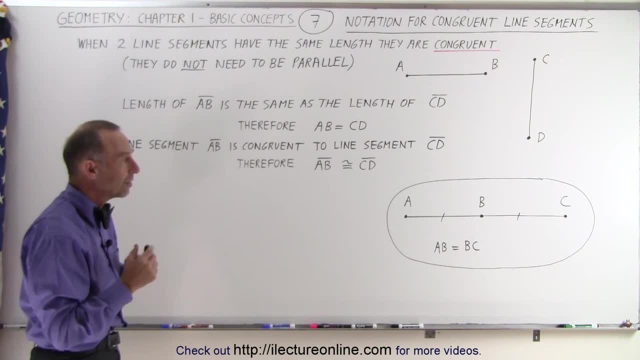 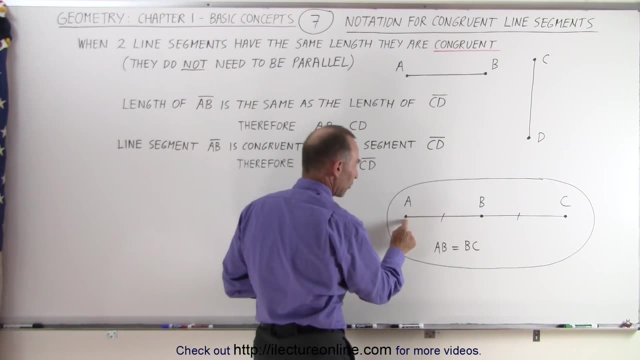 which we can write a notation where we can see two line segments being the same length is by making a little tick mark in there and a little tick mark in there. So here we can see we have a line segment from A to B and a line segment from B to C And again by inspection you can see they appear to be. 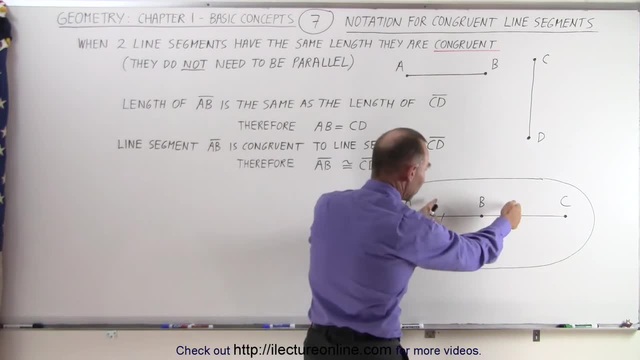 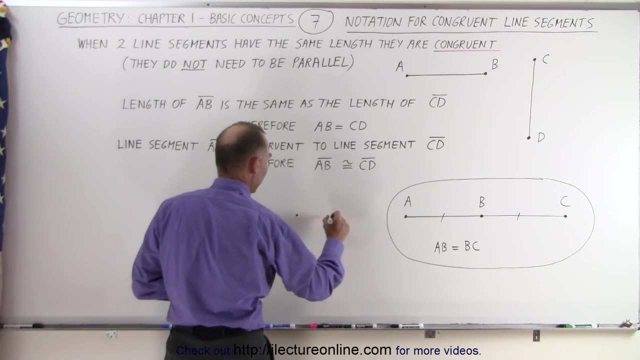 the same length. Let's show that they're the same length by making a little tick mark there. Then if we have another two line segments, let's say we have a line segment from D to E to F, for example, like this. So let's say: 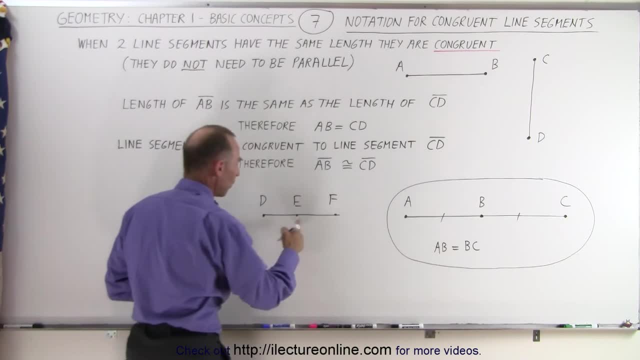 this is D, this is E and this is F. And if you want to show that the line segment from D D, E is equal to the line segment E- F, then we can put two little tick marks here indicating that these have. 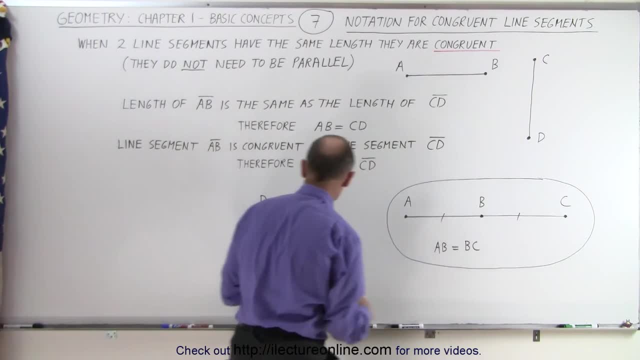 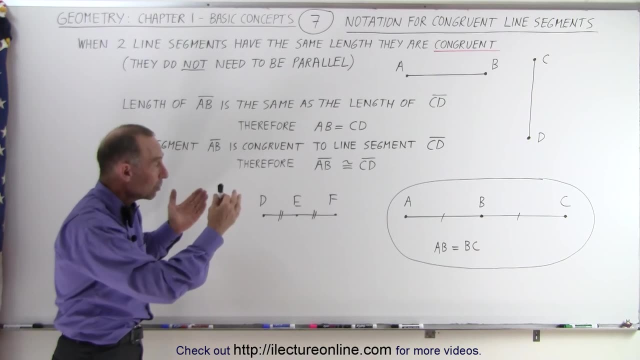 the same length and that these have the same length and that this length is not the same. So in this case we're going to do it differently. So we're going to use a little bit of different notation here to show that one of these lines is equal to the other line. segment.